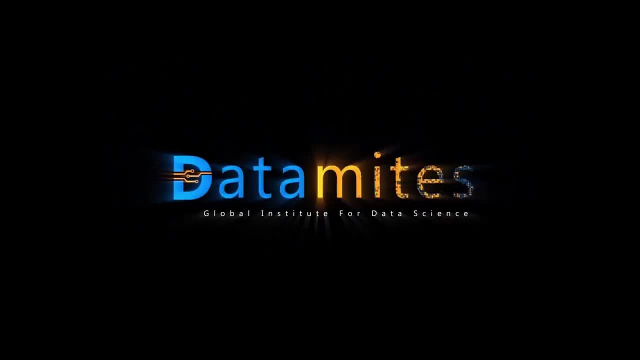 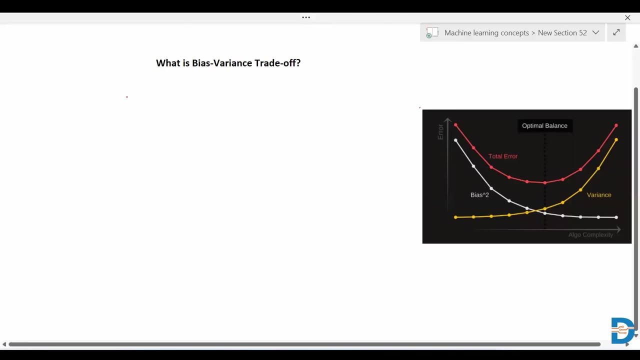 Hello everyone. So now we'll understand what is biased variance trade-off- Okay, So before that, we should know what is bias and what is variance. Okay, So bias and variance are very important parameters while training a machine learning model. Okay, So these can be considered as: 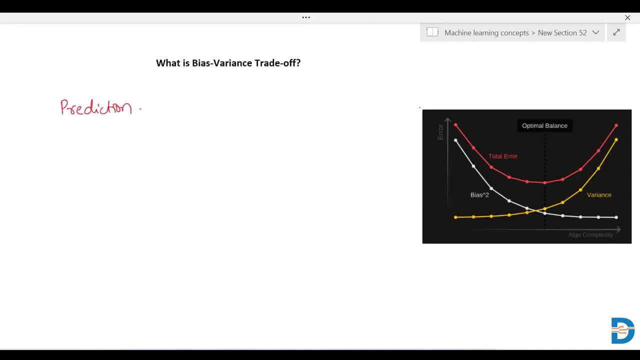 prediction errors. Okay. So what is bias? basically, Bias is distance between: distance between the predicted value, distance between the predicted value and the actual value. So this is the distance between the predicted value and the actual value, Or you can say the true value. Okay, So in this type of error. or you can say in bias. 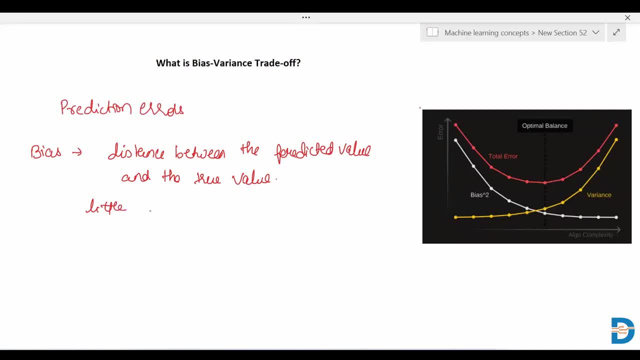 the model pays very little attention to the training data. Little attention to the training data, Okay, And oversimplifies the model. Oversimplifies the model, Okay. While in variance, variance, what is variance first? Variance tells us the spread of our data, Okay. Variance tells us the spread of our data, Okay. So in variance, when the variance is high, it pays lots of attention to the training data. It pays lots of attention, Lots of attention, to training data, Okay. 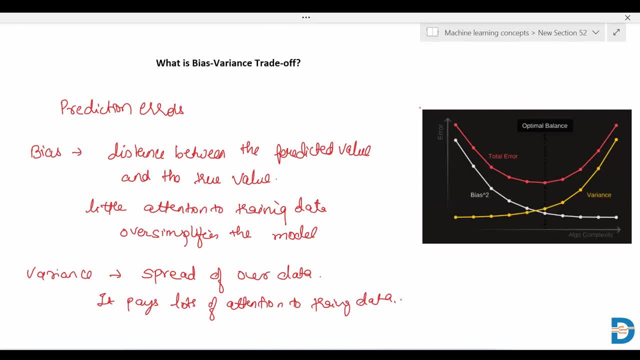 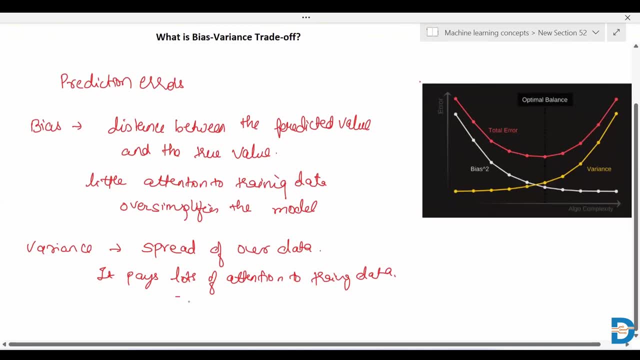 So such model performed very well on training data, but has high error rates on the testing data- Okay, Good performance on Good performance on training data: Okay, but high error rates. high error rates on testing data- Okay, Okay, Okay, Okay.